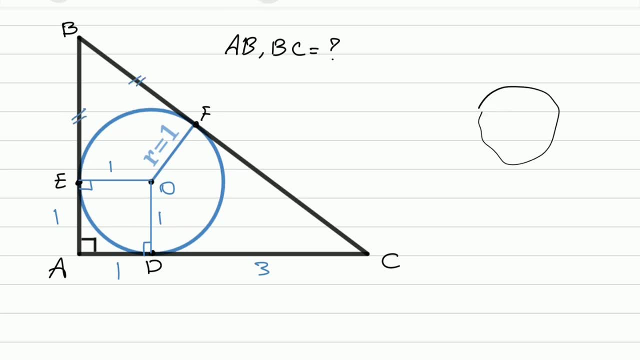 AE and BF are of the same size. Actually, it's a general rule, It's a theorem and it says: if you draw two tangents from a point outside of a circle to the circle, the length of the two segments are the same. 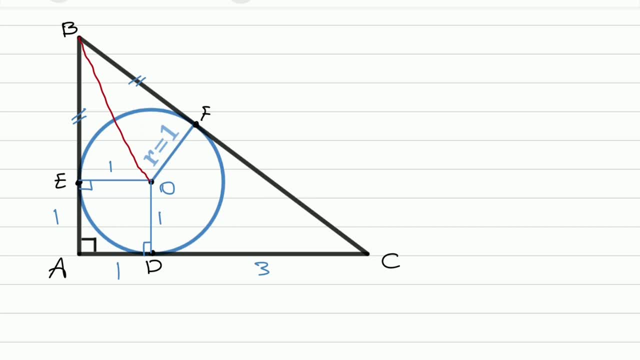 In order to do that, I'm going to draw the segment BO. and now I'm going to use the Pythagorean theorem a couple of times. First, on the triangle: BEO, So BE squared Is BO squared minus OE squared, And OE is the radius of the circle and it's equal to OF. so that's equal to BO squared minus OF squared. 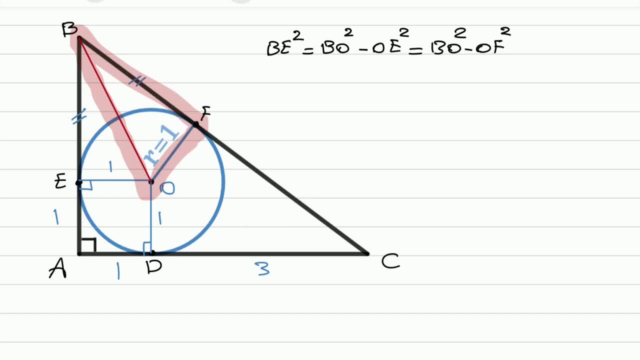 Now take a look at the BOF triangle and according to the Pythagorean theorem, BO squared minus OF squared is equal to BF squared. This is what we needed to prove. BE equals BF, And we're going to call that X. Now the same thing happens for the tangents from the point C. 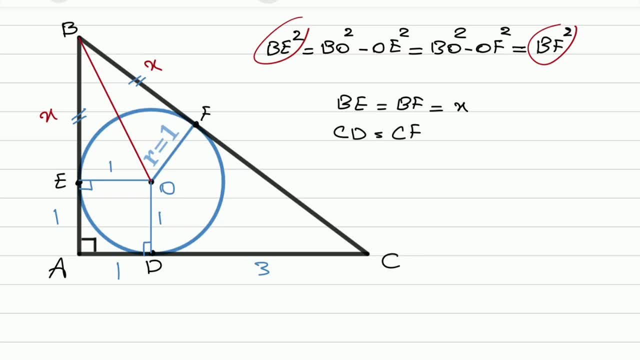 That means CD equals CF equals to 3.. So let's write it here: CF is equal to 3.. And also from the point A, AD is equal to AE. but we have calculated that from before and it checks here: AD and AE are equal to 1.. 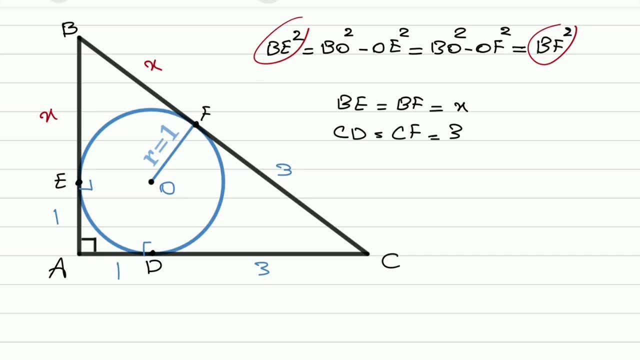 Now we're going to make one last move here and solve the problem. We apply the Pythagorean theorem on the triangle ABC. So BC squared equals AB squared plus AC squared, and BC is X plus 3.. AB is X plus 1 and AC is 4.. 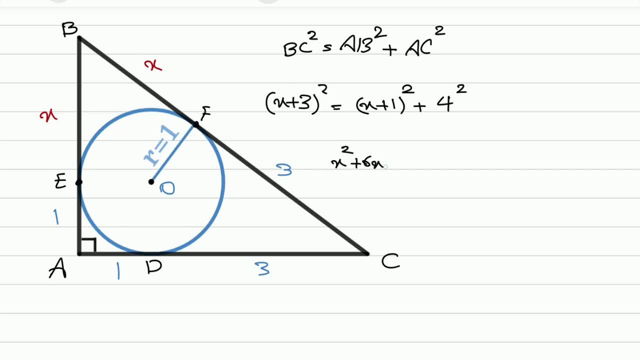 Now we expand it: X squared plus 6, X plus 9, and on the right side we have X squared plus 2, X plus 1 plus 16.. Powers of 2 cancel out and it makes it really simpler. 4 times X equals 8 and X is equal to 2.. 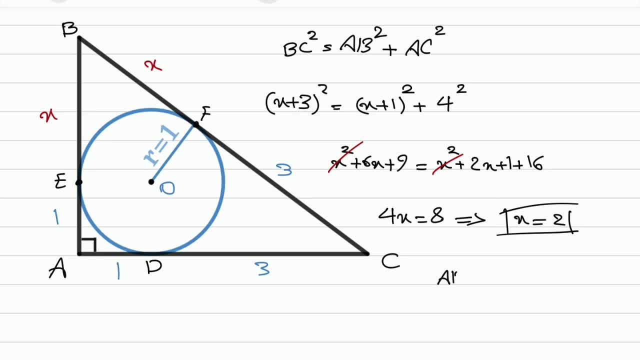 That's not the final answer. AB is X plus 1.. That's 3.. And BC is X plus 3. And that's 5.. Now, this is the final answer, And this is the end of this video. Take care Until the next one. See you soon.